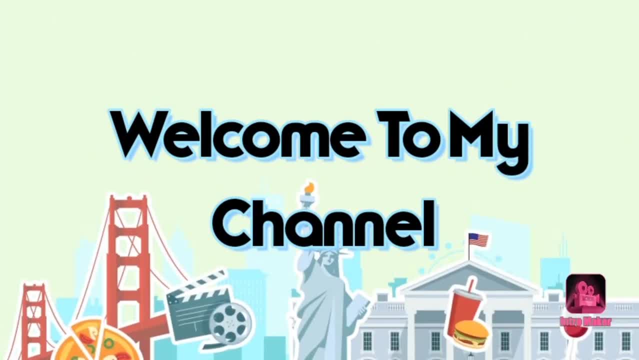 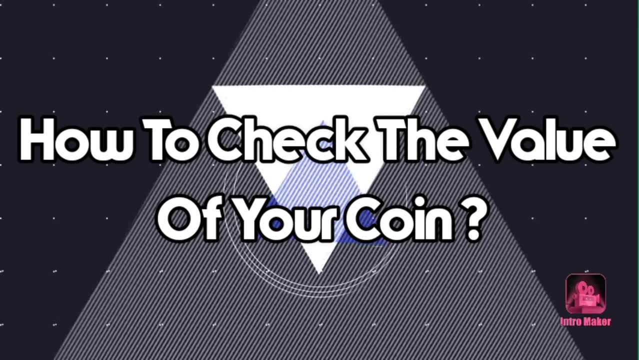 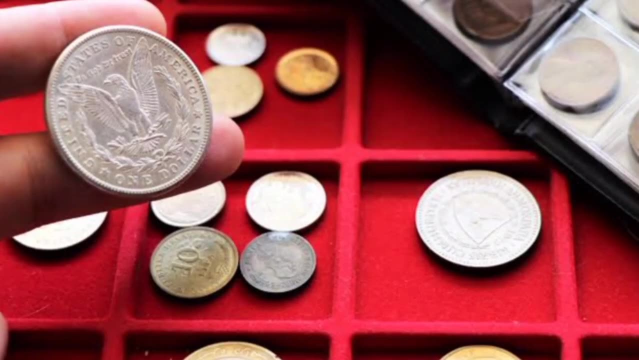 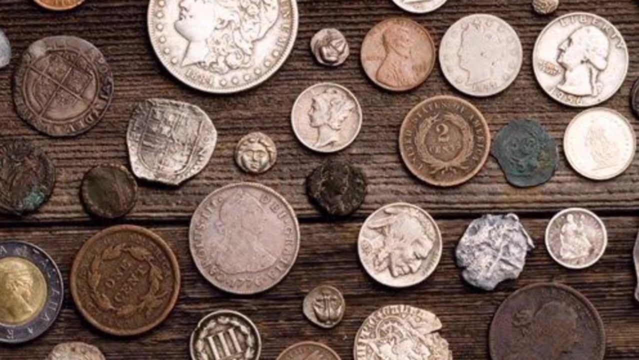 Welcome to my channel, Jags Rocks. How to check the value of your coin, How to find the value of old coins. Coin collecting is a fun hobby, but collectors naturally want to know the value of their coins. This can be out of curiosity or because they are interested in coins for investment purposes. 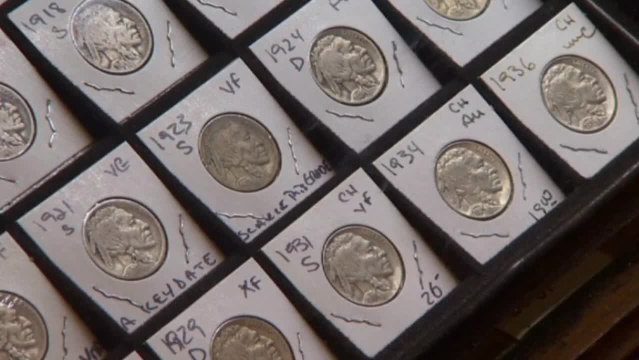 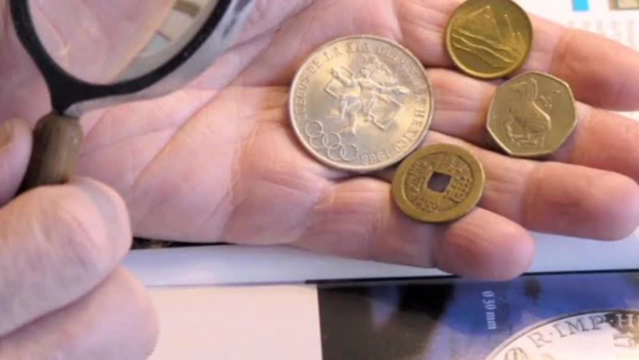 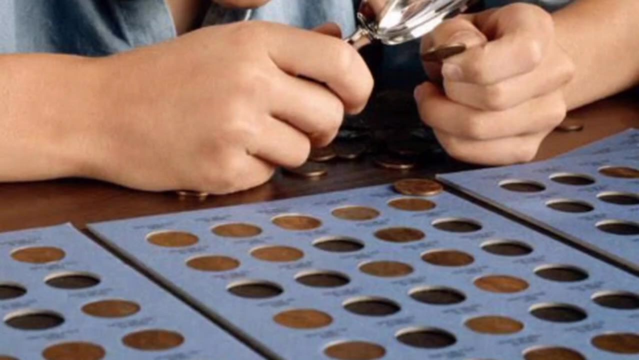 Whatever your reason for collecting, start by figuring out exactly what type of coin you have, as well as its condition. You can then reference this information against online and print value lists If you want to get an accurate value for your specific coin. work with a numismatics organization and the Professional Appraiser Method 1 of 2.. 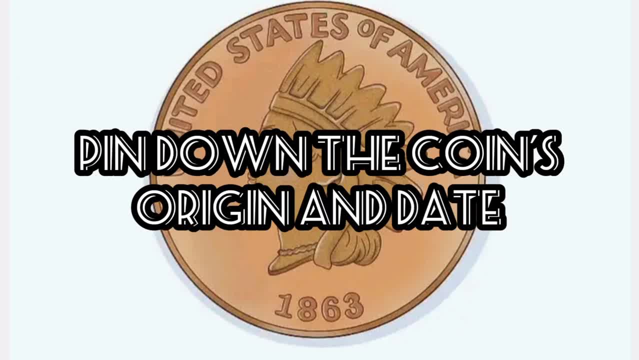 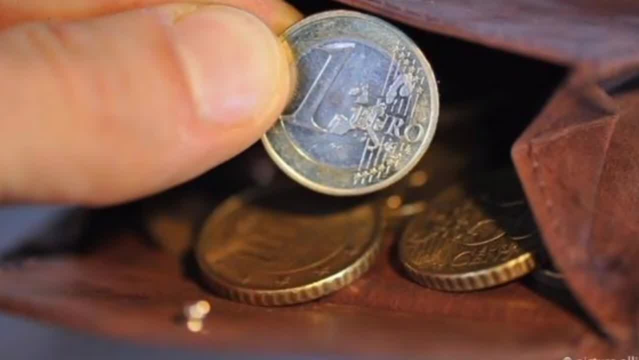 Research number 1: Write down the coin origin and date. You'll need to know exactly what coin you're looking at to determine its specific value. Modern coins will include a date of issue printed on the front or back of the coin itself. They will probably also name the country of origin. 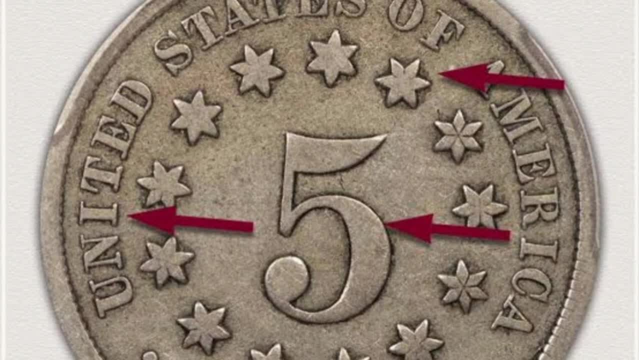 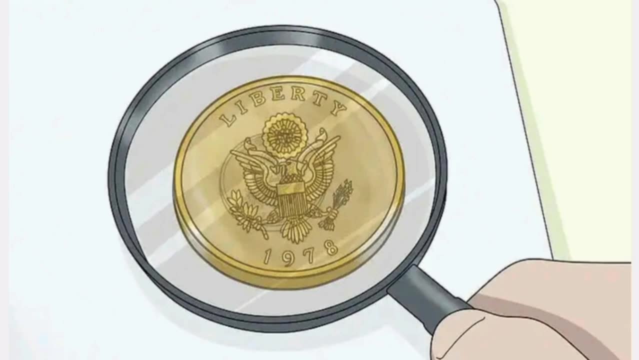 Some also have other helpful information, such as a mintmark, a tiny letter printed somewhere on the coin that indicates where it was minted. If the information printed on the coin is printed in the language you can read, you'll need to look at the coin reference book or website. 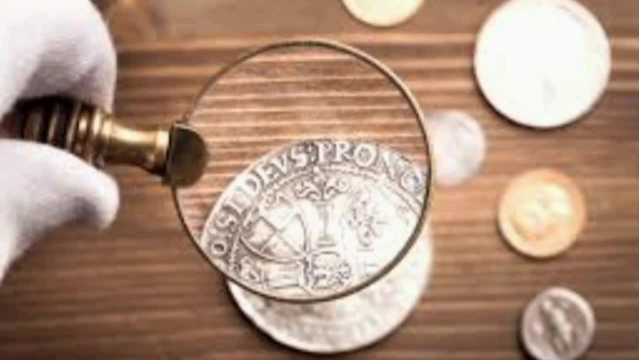 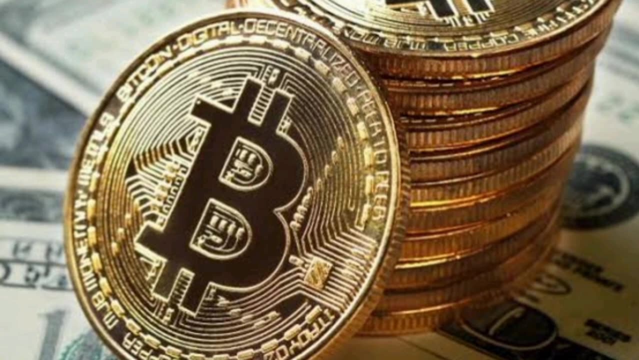 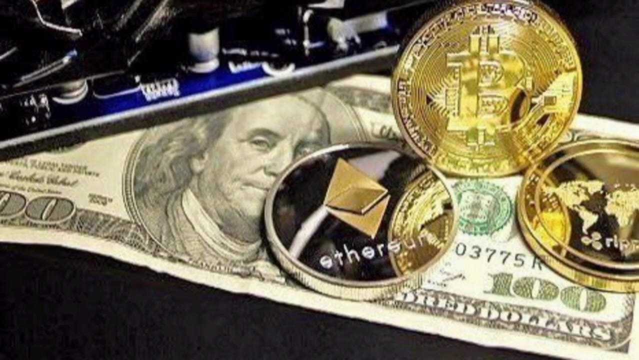 These will include images that will help you match your coin. These guides can also be used to help you determine how old coins without a printed date are. If you cannot find the coin in a book due to lack of identifiers, try to determine general area, that is, Sinosphere, Islamic countries or African. 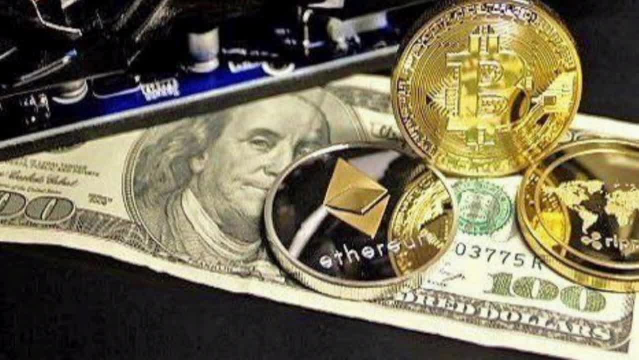 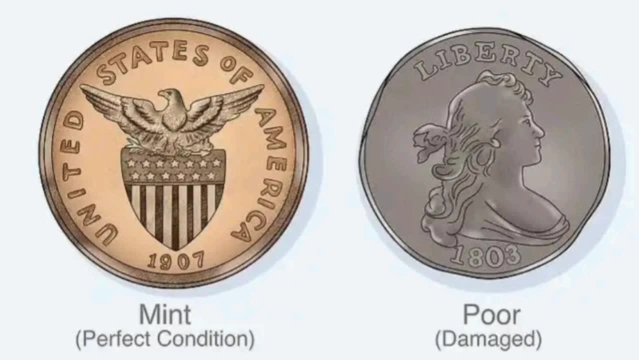 Broadening your search first may help you narrow in on the correct country. Number 2: Expect the coin to determine its condition. The value of a coin is greatly affected by its condition. Higher quality coins are generally more valuable than ones that are blemished or dirty. 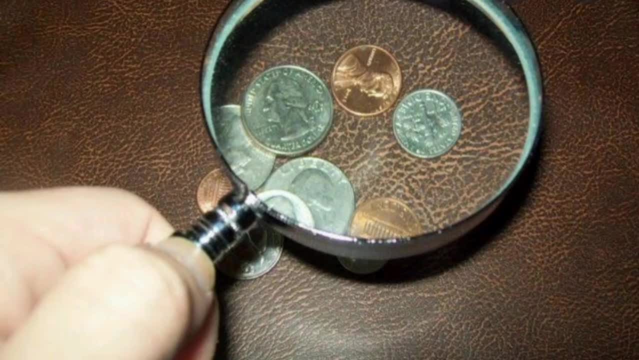 Coins that were never used are known as uncirculated Coins are rated from imperfect condition all the way down to were dirty or damaged. If you have a coin that you think might be rare or valuable, don't attempt to clean it yourself. 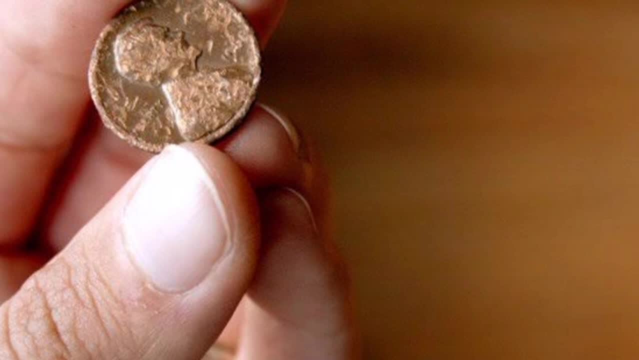 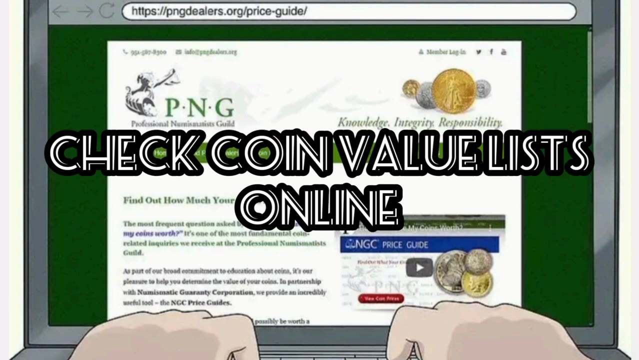 Take it to an expert to have it cleaned without damaging it and leave it. If a coin is severely damaged, it might just be worth the value of the metal itself. Number 3: Check coin value lists online. Some websites will make values for some coins freely available. 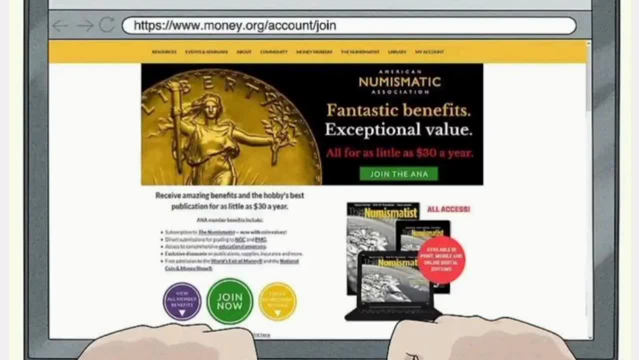 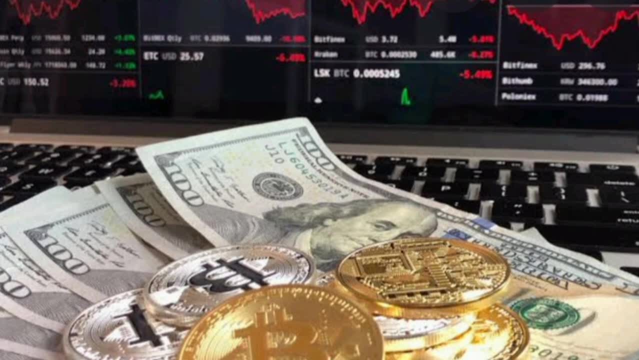 Check with a professional organization like the Professional Numismatics Guild. Look up your coin according to its date and origin and you may be able to find its current value. A number of factors, including condition and current demand, impact the amount a coin can have. 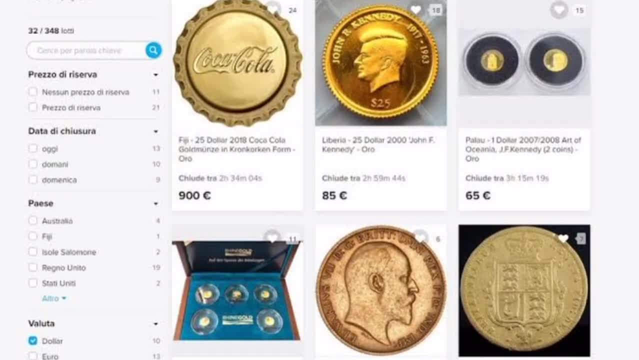 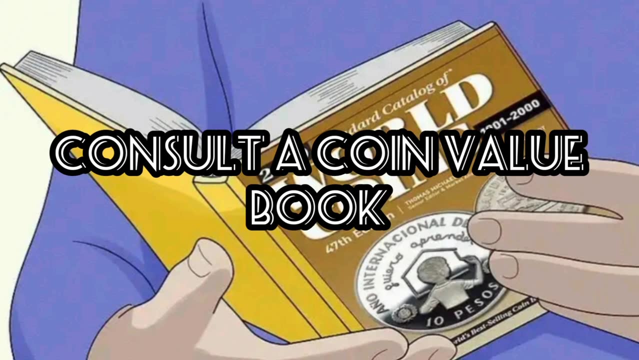 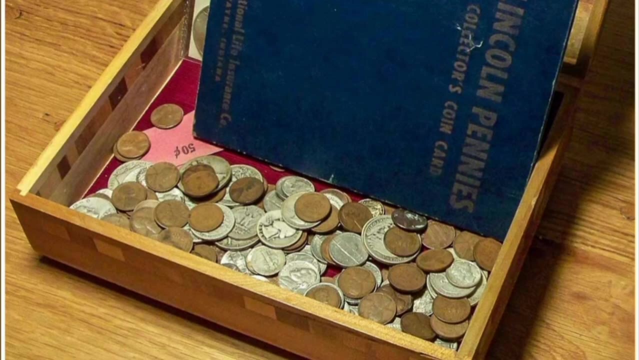 If a coin is actually sold for, so use the value you find online only as a ballpark figure. Number 4: Consult a coin value book. If you can find the value of your coin online, consult a reference such as the Standard Catalog of World Coins or the Guidebook of United States Coins. 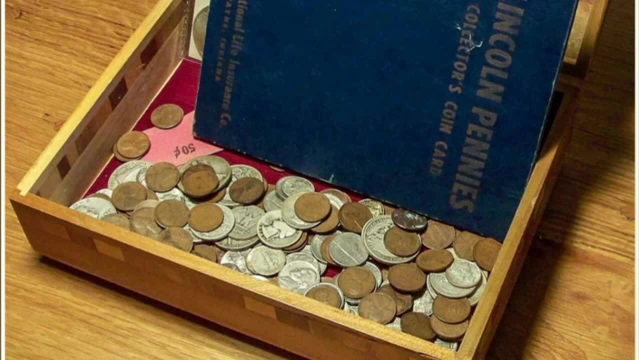 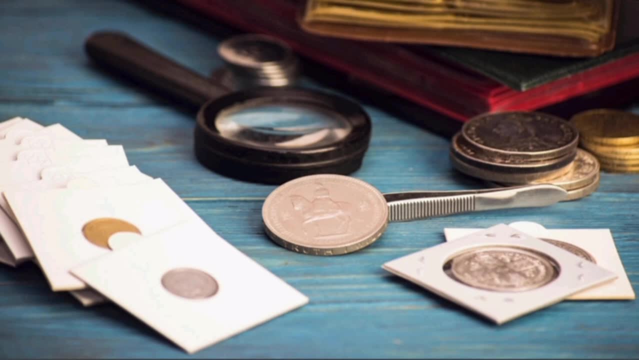 These references are especially useful because they may list several values for a particular coin: The UIC value, a generally accepted value of the coin. The UI value: what a dealer would pay to buy the coin from you. The retail value: what a dealer would sell a coin to a customer for. 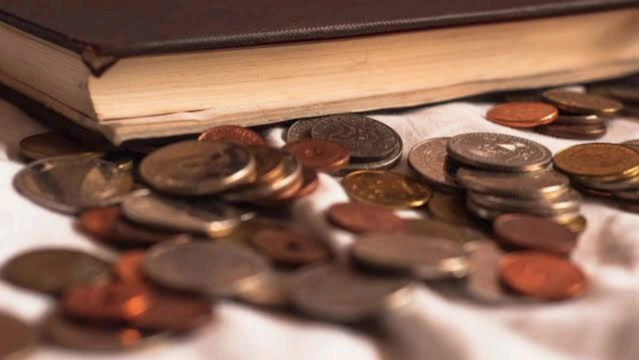 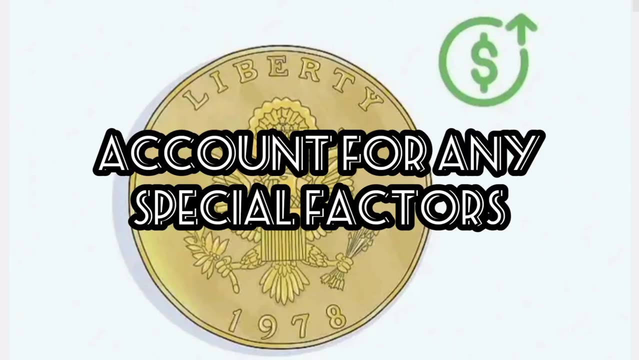 The wholesale value what a dealer might sell the coin to another dealer for, especially when several coins are sold together. Number 5 Account for any special factors. The value of coins can go up and down, since they are driven by interests that can change. 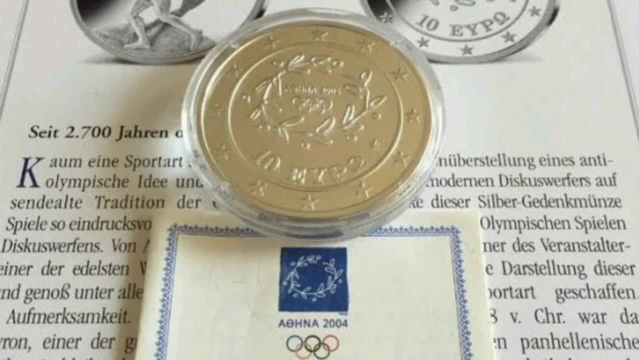 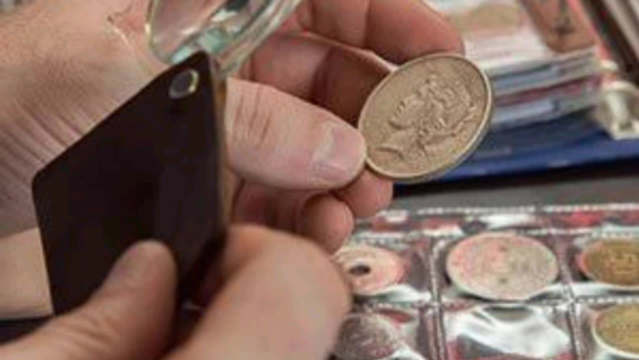 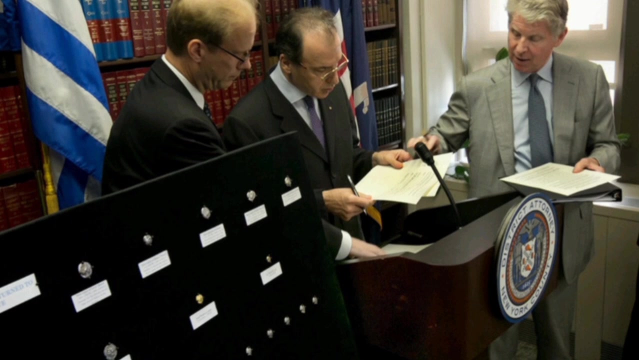 When lots of people want to buy a certain type of coin, the value may go up. Rare coins or coins in unusually fine condition are often more valuable than common ones. Finally, commemorative special issue coins may also be especially valuable. Take these values into account when calculating the value of your coin. For instance, you may have a type of coin that is not especially rare. However, if it is in mint condition- and most coins of that type are not- its value may be higher than the normal UIC value method 2 of 2.. 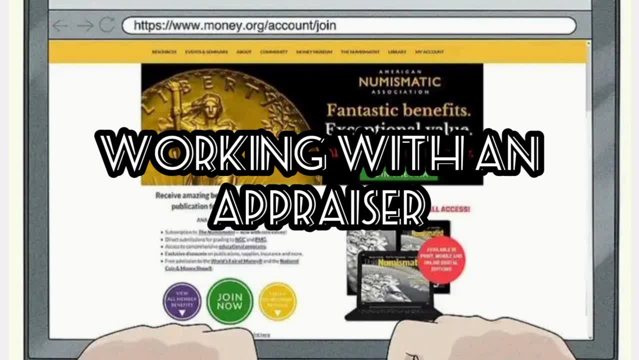 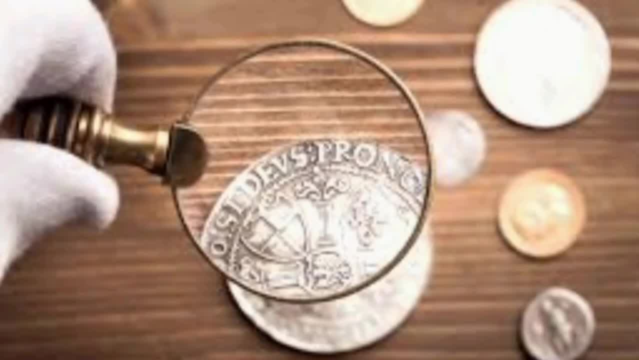 Number 1: Working with an appraiser. join a numismatics group- The study of coins and other money is known as numismatics- If you have lots of coins that you want to appraise or if you frequently work with coins. 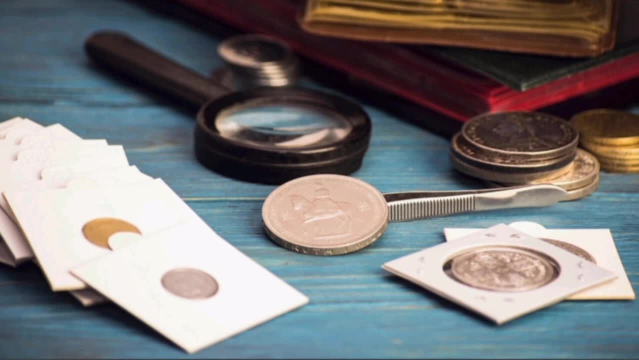 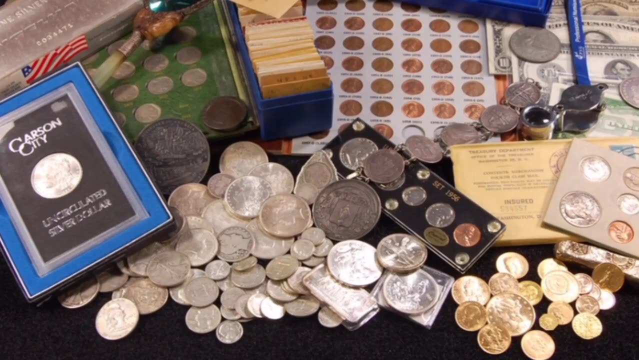 consider joining a professional group devoted to this area. These groups will share price lists and other special information that can help you determine the value of your coins. Look for a recognized professional group in your area, like the American Numismatics Association or the Professional Numismatics Guild.